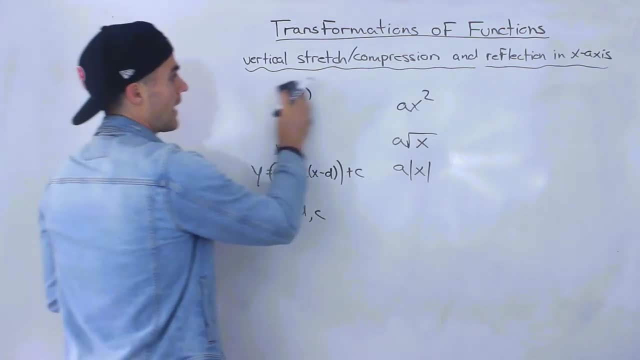 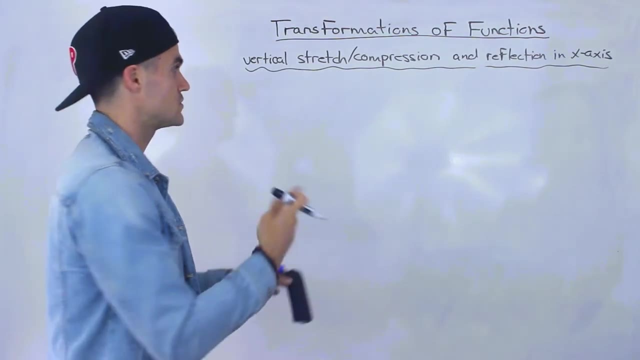 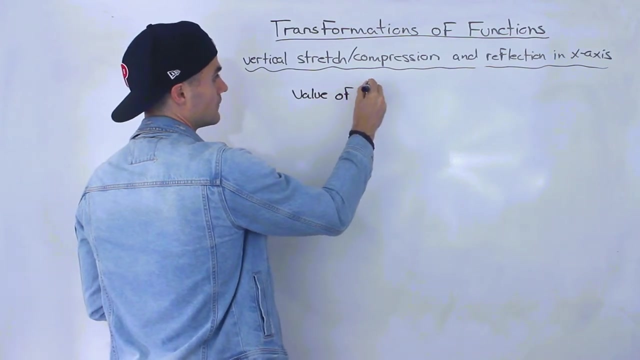 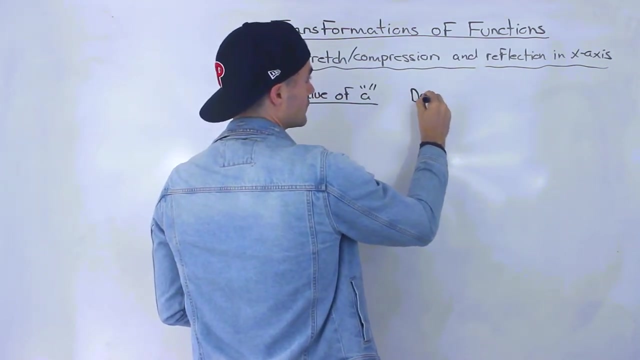 usually in front of the function And, depending on the value of a, the transformation is going to differ. So what I'm going to do is I'm going to go over a couple of cases for the value of a That a can take, And then I'm going to give a description depending on what that value is. 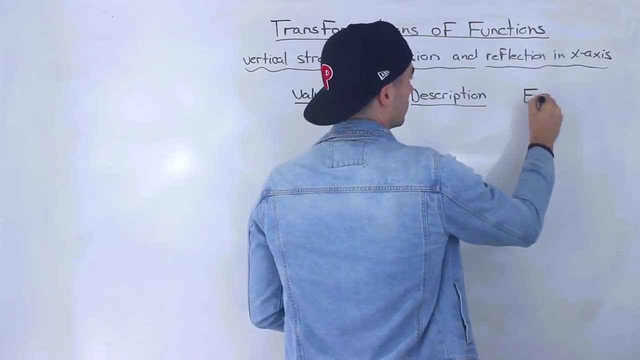 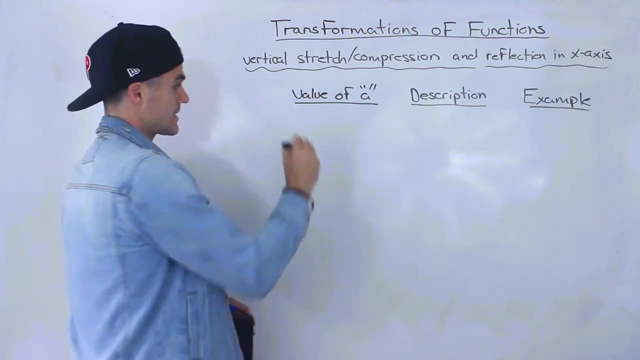 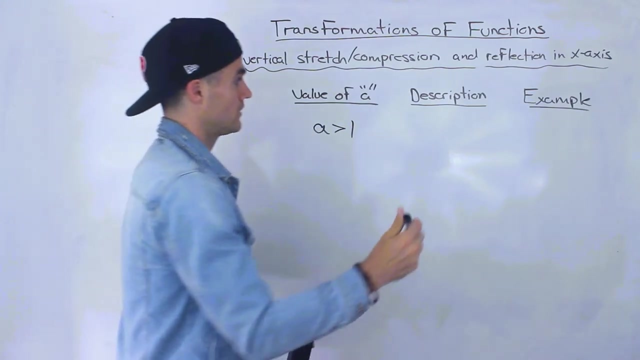 going to be, And then I'll show you an example Right. So the first case is if a is greater than 1.. So if the a value is going to be greater than 1, then what we say is that there's going to. 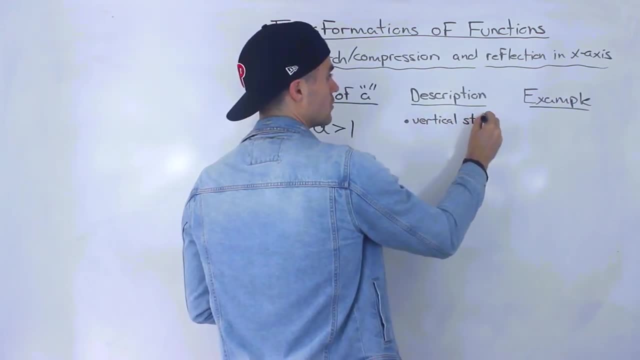 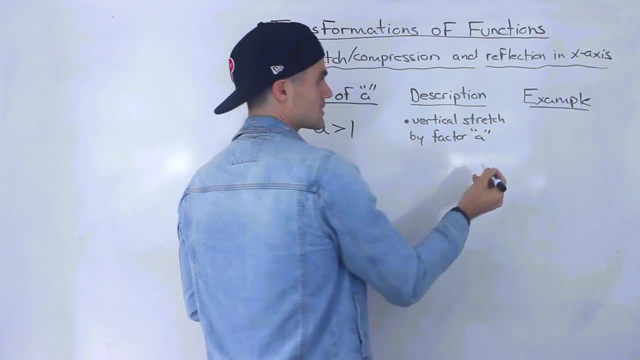 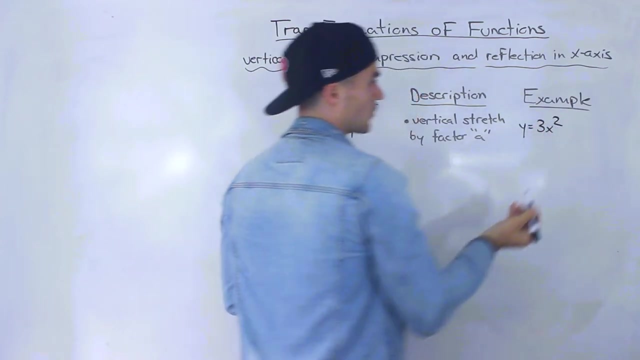 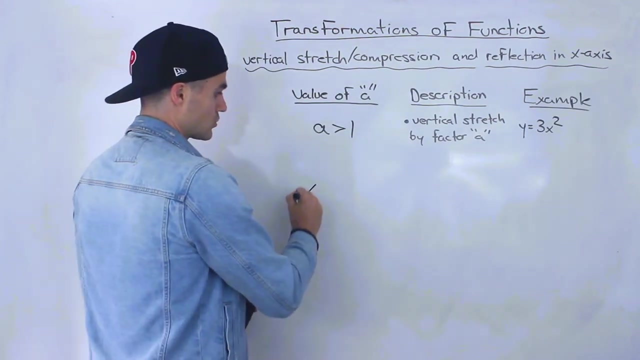 be a vertical stretch by factor a, whatever that a value is. So, for example, if we have y equals 3x squared, Notice that the a value is 3, so it's greater than 1.. So we would say that we took the function x squared and then vertically stretched it by a factor of. 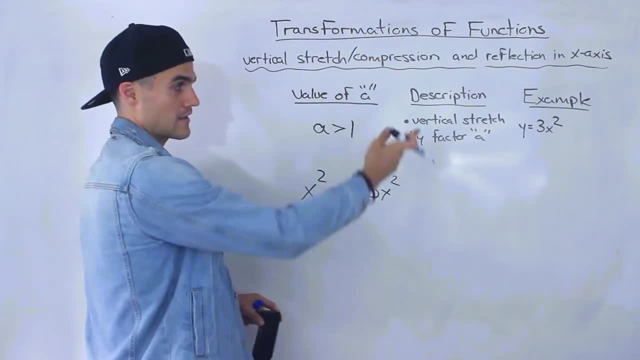 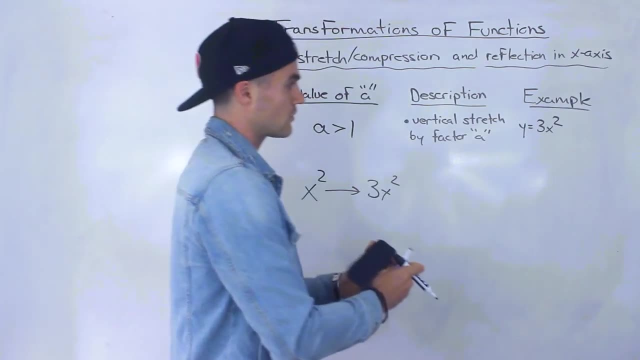 3 by that factor of a, In this case the a value is 3.. And the way this looks, I'm going to show you both x squared and then 3x squared. So the way both of these would look is: let's: 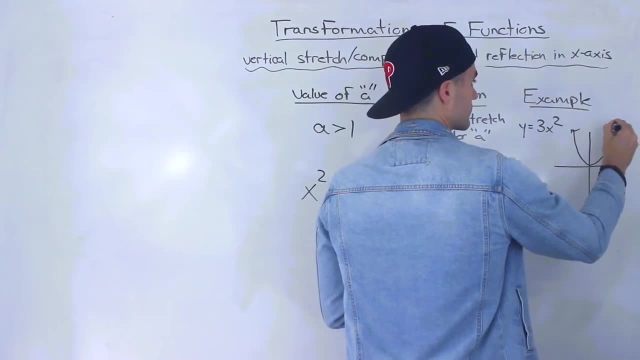 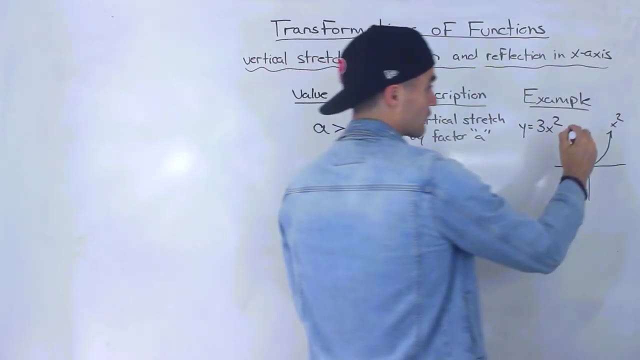 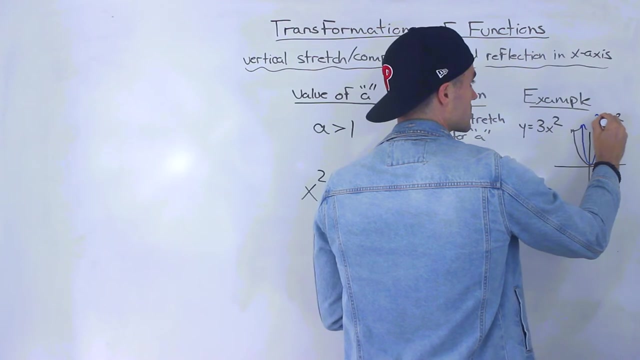 say, we have x squared here. Well, 3x squared. what's going to happen is we're going to take this and vertically stretch it by a factor of 3. And when we vertically stretch something, this is what happens. So that's how 3x squared is going to look compared to x squared. So notice it becomes. 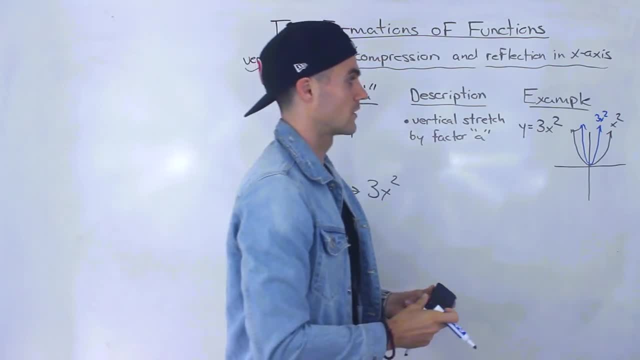 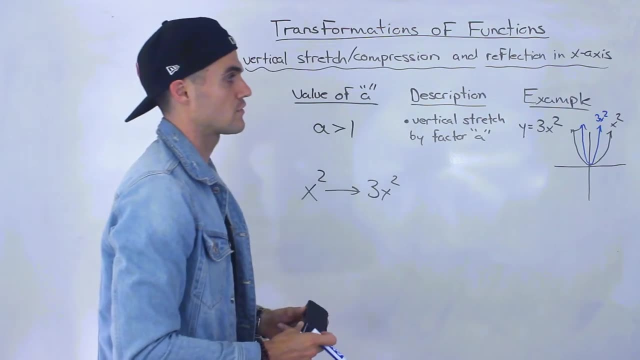 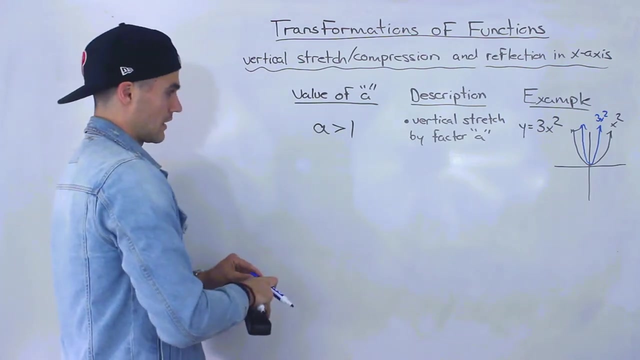 more thinner and higher as well. Just took this x squared and vertically stretched it, and in this case by a factor of 3. So that's an example of a case when a is going to be greater than 1.. Now the next case is in. 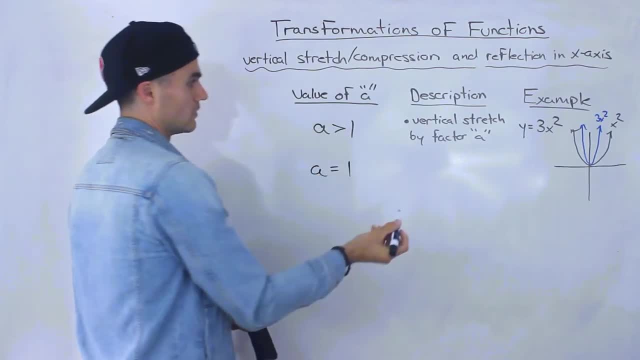 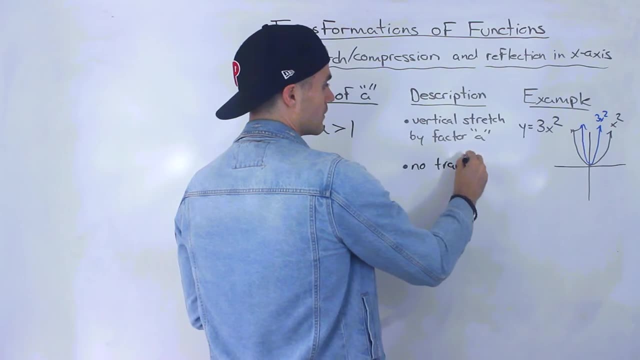 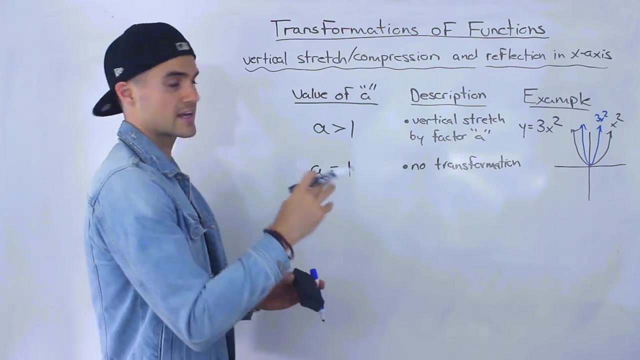 If a is equal to 1.. And if a is equal to 1, there's actually no transformation, Because if you think about it, it would just be 1 times x squared, which is just x squared. So that means x squared did not change. There was no transformation if a is equal to 1.. 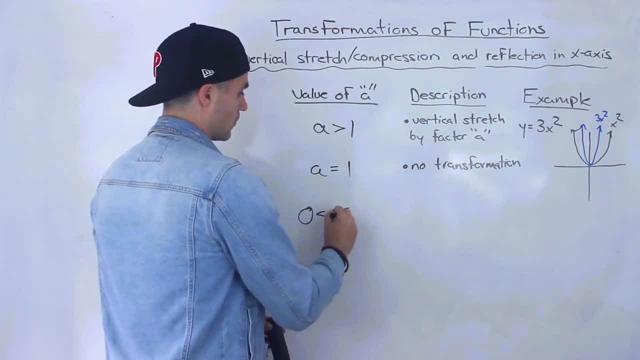 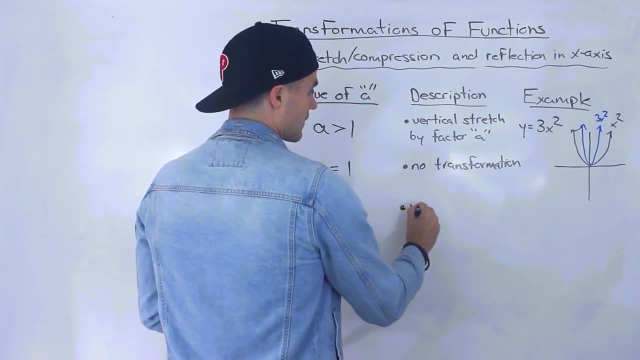 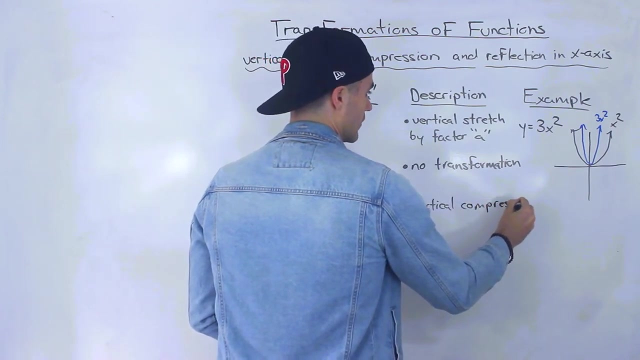 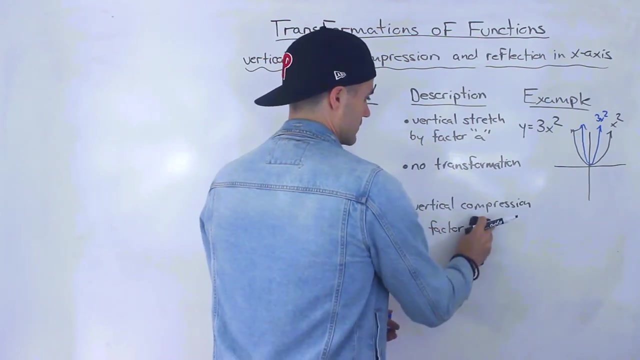 What if a is between 0 and 1?? What if a is between 0 and 1?? If this happens, If this happens, If this happens here, then we would say that there's a vertical compression by factor a. Sorry, let me put that a here in quotations Like that. 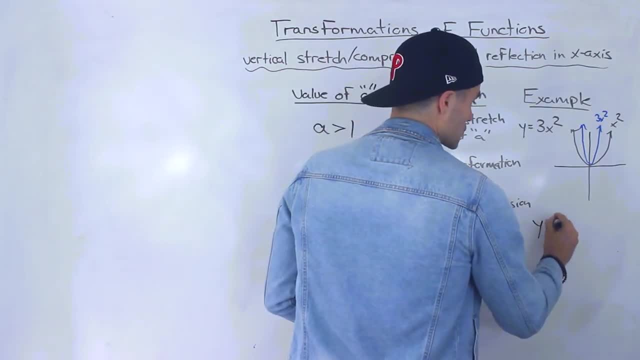 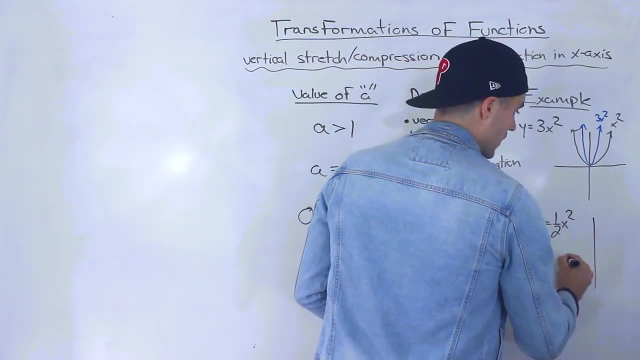 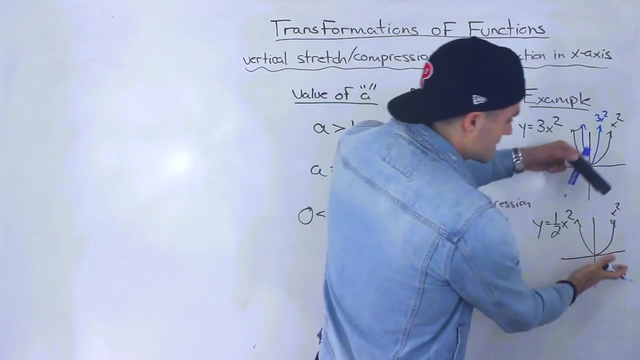 So an example of that is if we had maybe y equals 1 over 2 x squared. Okay, if we have y equals 1 over 2 x squared. here's how x squared looks like. But if we take this and we vertically compress it, then y equals 1- half x squared is going to be out here. 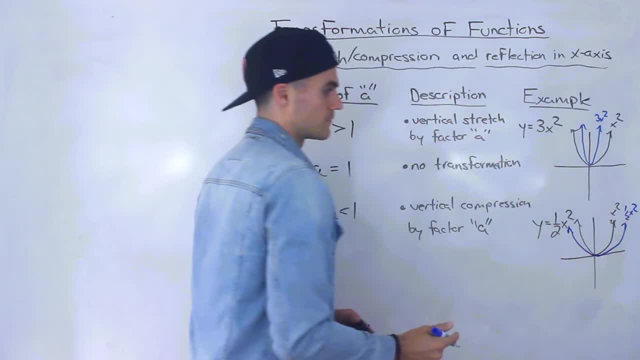 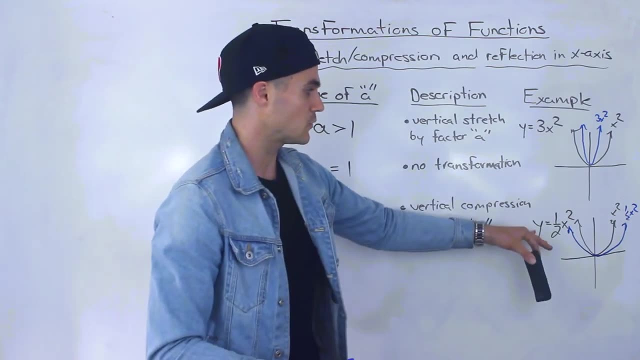 So that's going to be 1 half x squared. So it's going to widen the function Right And in this case, specifically, y equals 1 half x squared. Notice that the a value is a half, so it's between 0 and 1.. 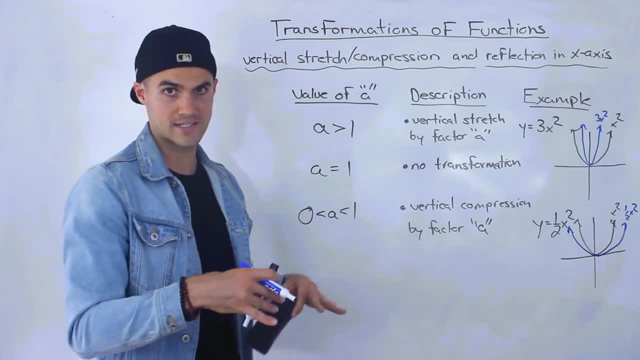 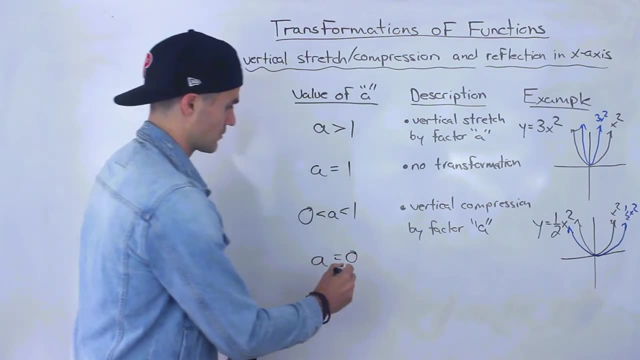 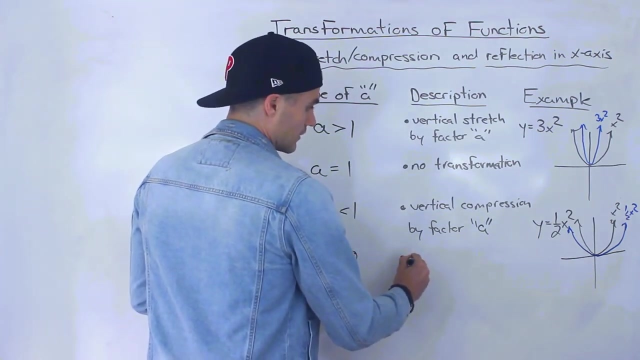 So we would say that x squared, is vertically compressed by a factor of 1 half. Now what if a is equal to 0?? So, following this kind of order, next up is 0.. Well, if a is 0, notice that there's going to be no function. 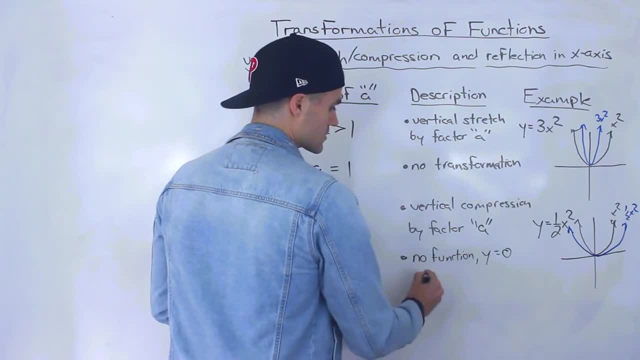 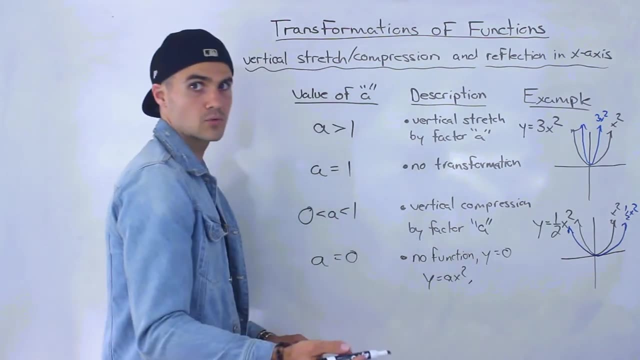 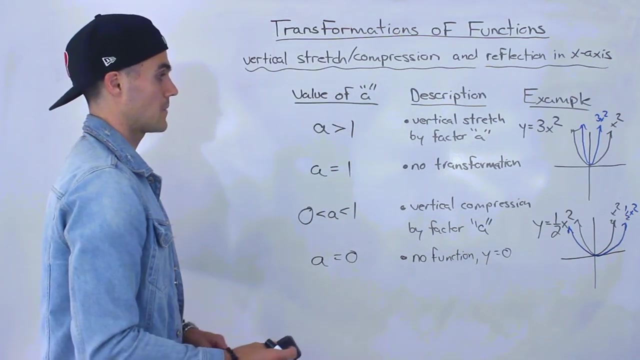 We'll just end up having y is equal to 0. So if we have y, y equals a x squared, that a value is 0. We just end up with y is equal to 0.. Right, So usually this case here will not come up. 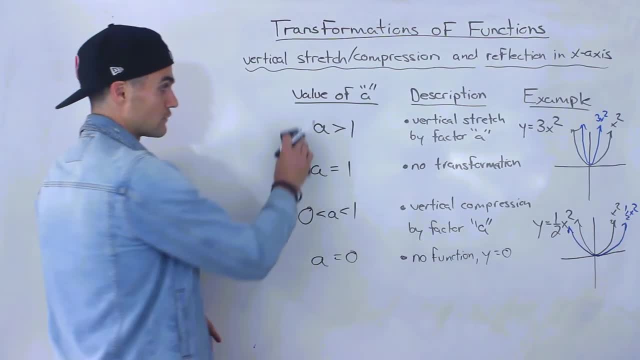 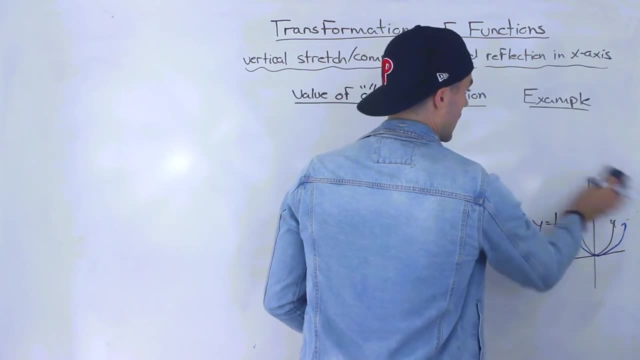 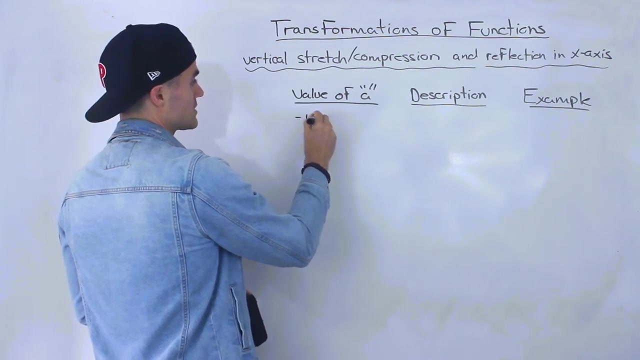 Right, And then after 0, what happens? We're going to get into the negative numbers now. So let's do a couple of cases with some negative values. So let's say that a is between negative 1, so it's greater than negative 1, but it's less than 0.. 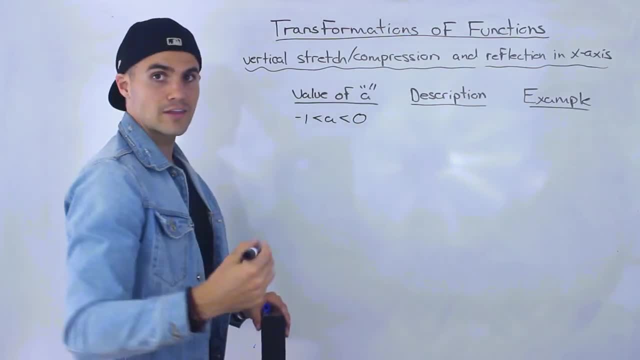 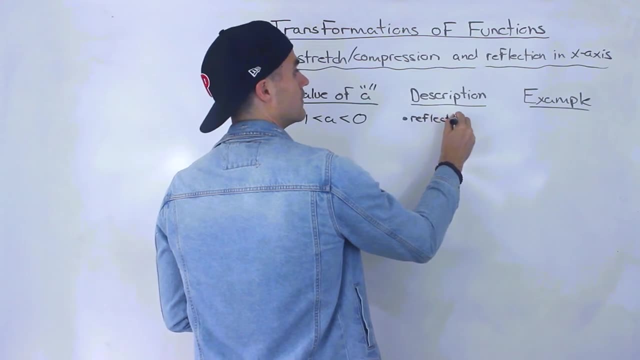 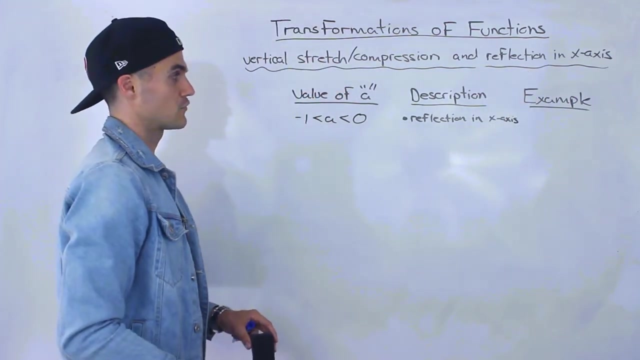 Okay, Whenever the? a value is negative, there's going to be a reflection in the x axis. So that's where that reflection in the x axis is coming from. Alright, So notice here If a is between negative 1 and 0.. 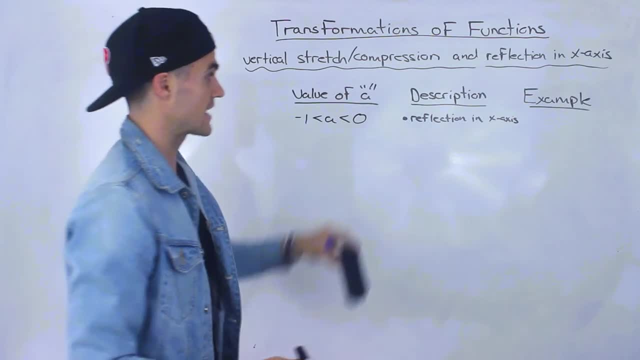 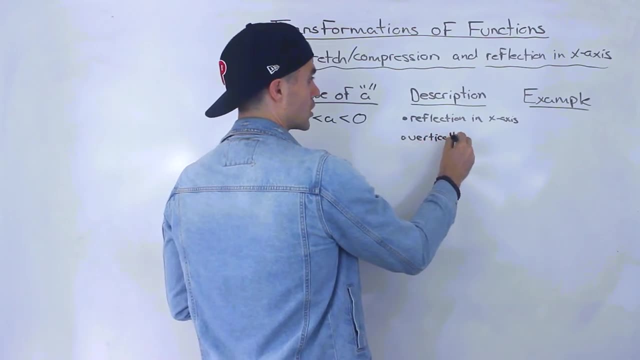 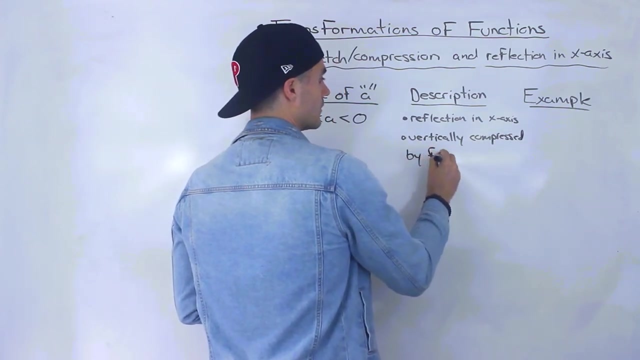 It's going to be a reflection in the x axis- be negative. so there's going to be a reflection in the x-axis and also in this case it will be vertically compressed by factor and we wouldn't say the a value, we would say the absolute value. 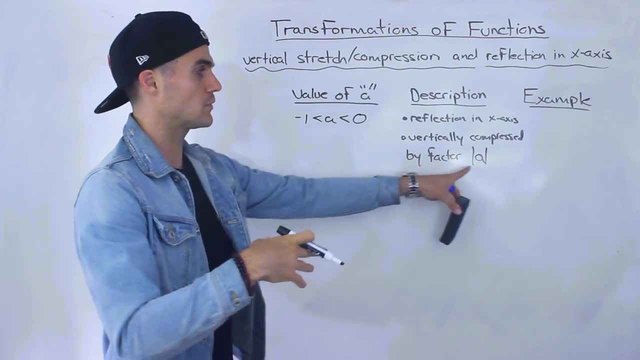 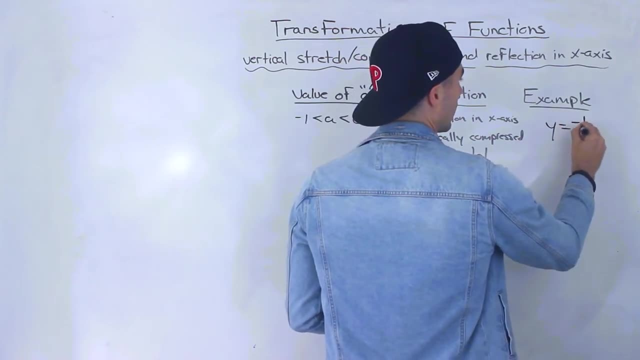 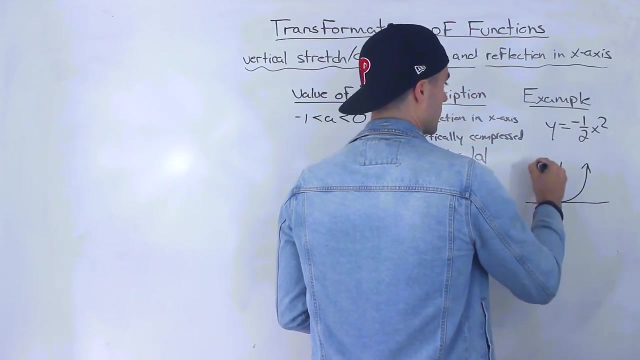 of a, because a is going to be negative. but when we're talking about a factor, we always mention the positive number. okay, so let me give you an example. let's say that we have y equals negative, one over two x squared, so let me draw both here. this is going to be x squared, well, because a is. 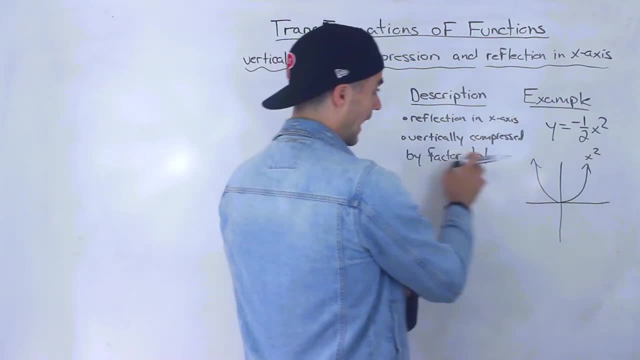 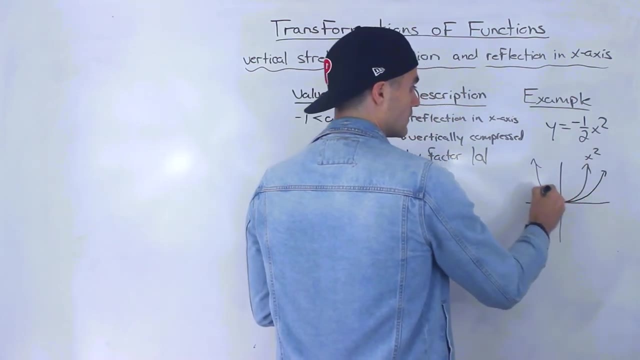 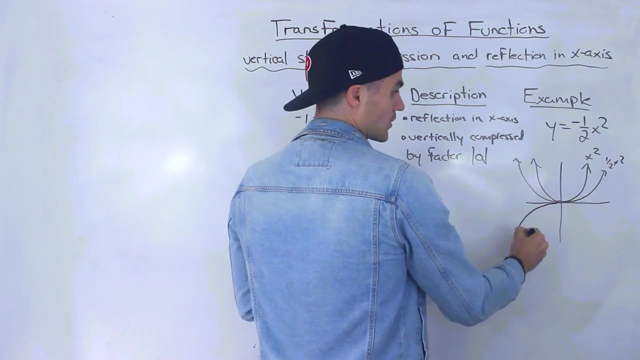 negative. there's going to be a reflection and there's going to be a compression. so remember that y equals one half x squared. look like this: it was wider. well, now what we're going to do is we're going to take that wider function. we're also going to 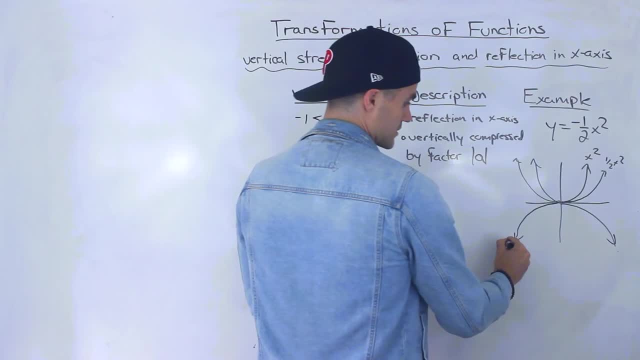 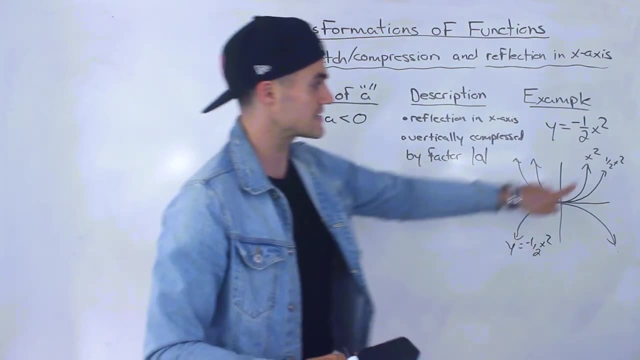 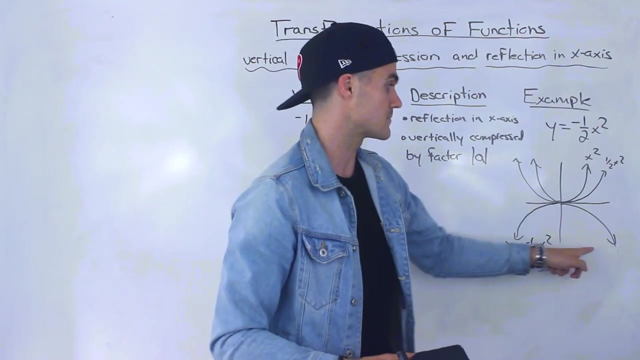 reflect it. sorry, i should have put this in a different color. it's all good, so this would end up being negative one half x squared, so it's the exact same as half x squared, except it's reflected now in the x-axis, so it's pointing downwards, right? so if you got a function like this, 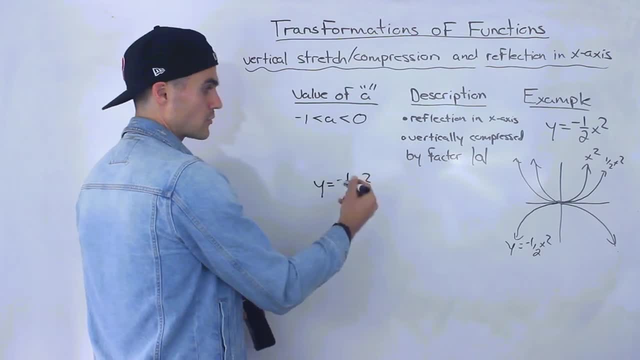 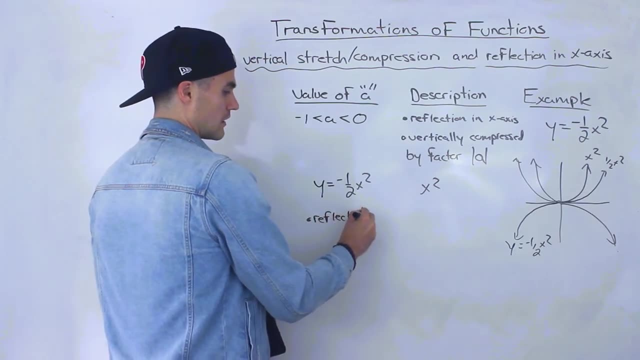 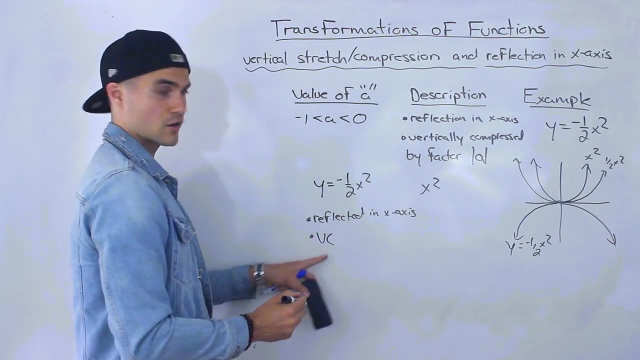 you're going to have a reflection in the x-axis and you're going to have a reflection in the x-axis and you have to describe the transformations from the parent function. x squared. you would say it's reflected in the x-axis and then it's vertically compressed. i'll put vc here for short form, vertically. 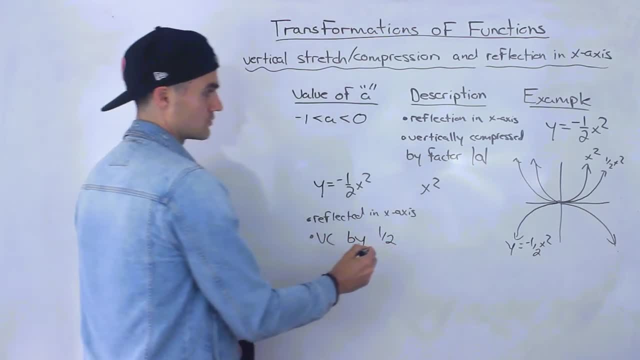 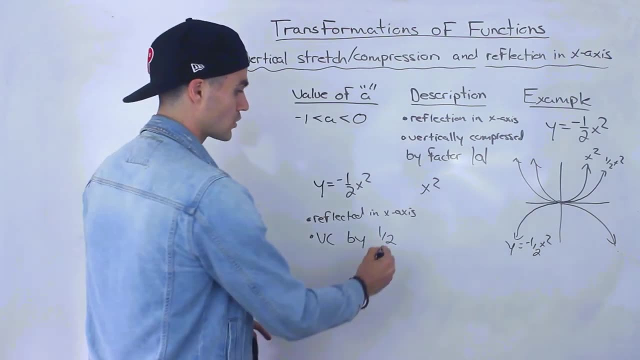 compressed by a factor of one over two, which the a value is negative a half. so the absolute value of negative a half is positive a half. right, whenever you're writing the factor of one over two, you're going to have a reflection in the x-axis and then it's vertically. 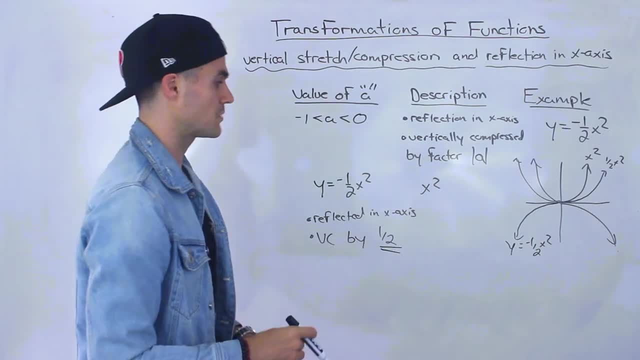 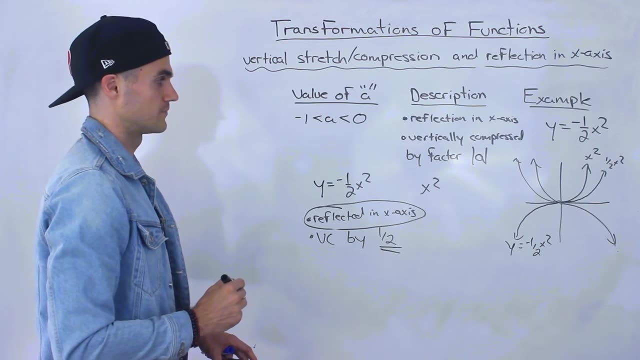 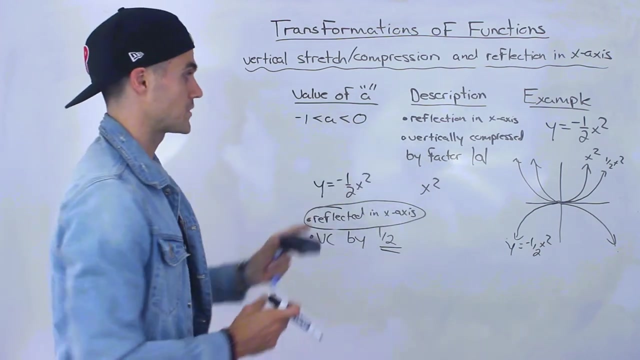 compressed by a factor. when you're describing the factor in words, you always put the positive value- the fact that it's negative gets taken care of in this description- in the reflection right. so if the a value is between negative one and zero, this is what happens now. what if the a 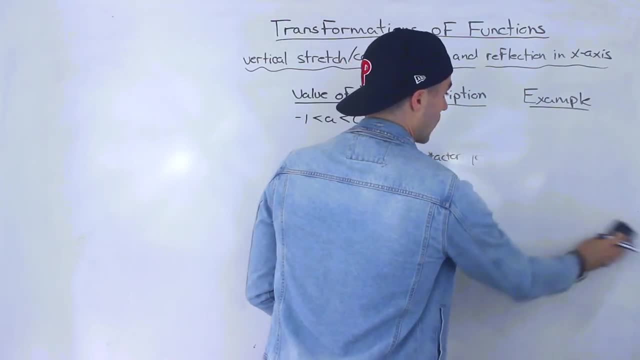 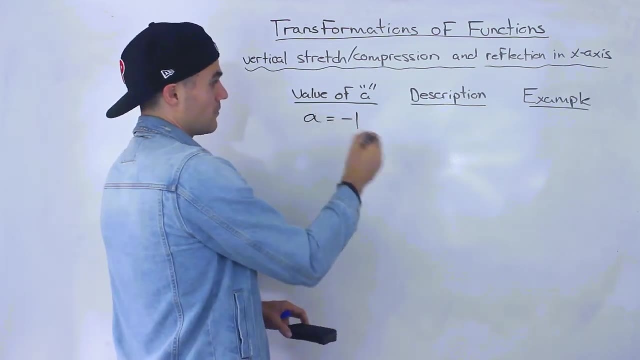 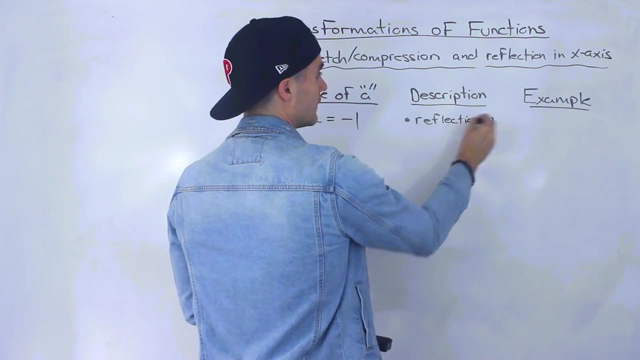 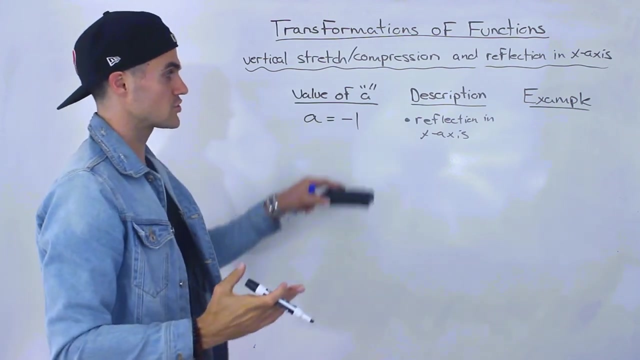 value is um is just negative one. remember, when the a value is positive one, we said that there is no transformation. but if it's negative one, there is a transformation and it's only a reflection in the x-axis. so in that case there would be no vertical stretch or compression, there's just a. 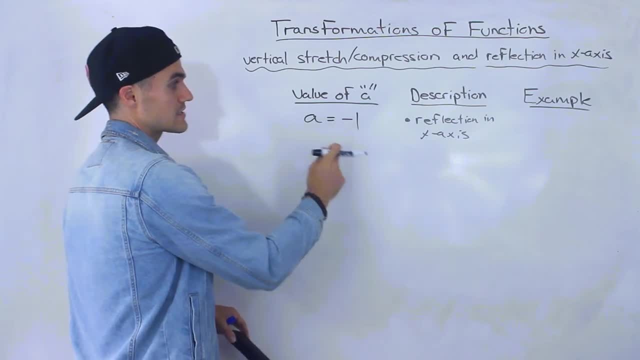 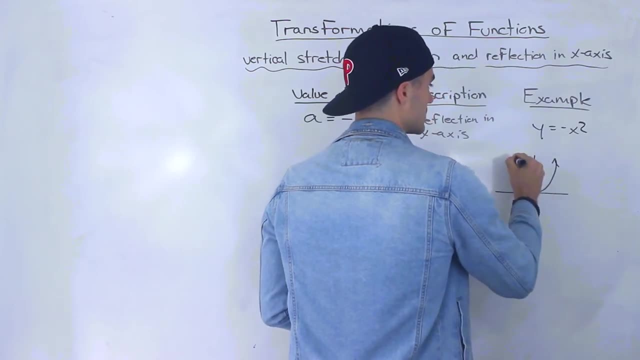 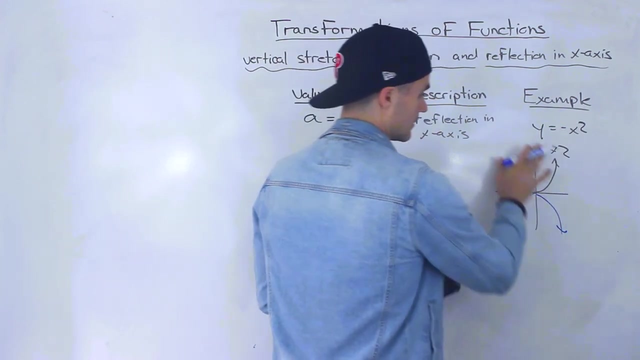 reflection in the x-axis, in the x-axis, if a is negative one. so if we have y equals negative x squared. well, x squared looks like this and negative x squared. it's just going to be reflected in that x-axis, so it's going to be pointing downwards. that's going. 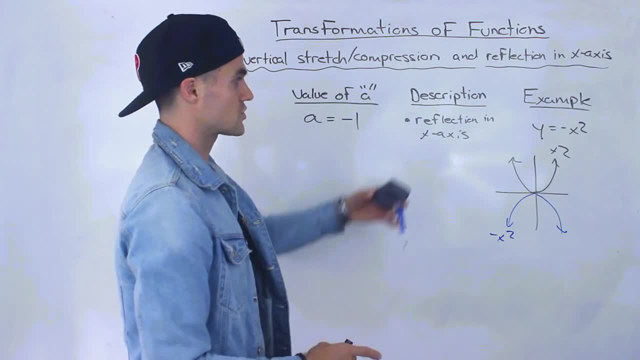 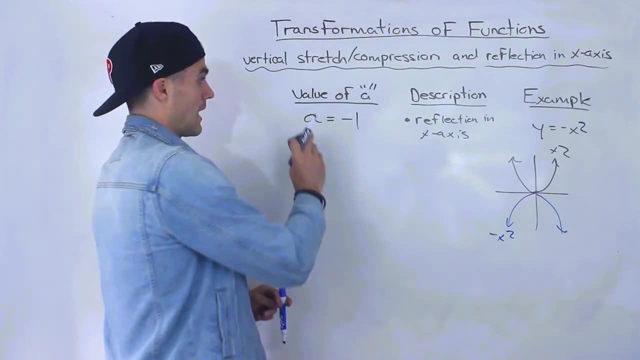 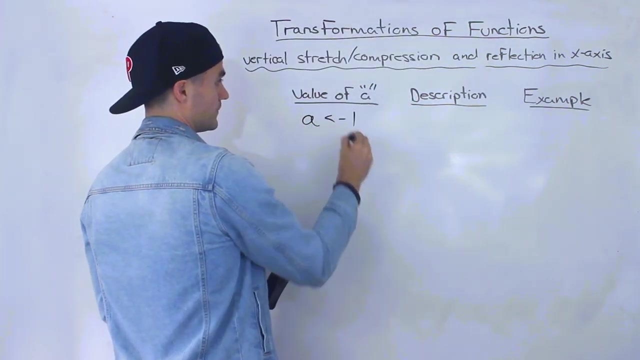 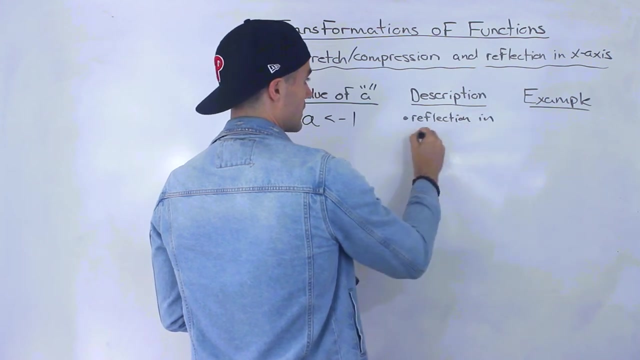 to be negative, x squared right. so there's just a reflection in the x-axis if a is negative one and there's no vertical stretch or compression. and then, finally, if a is less than negative one, then we say there's a reflection in the x-axis because it's still negative and we would say there's a vertical stretch.